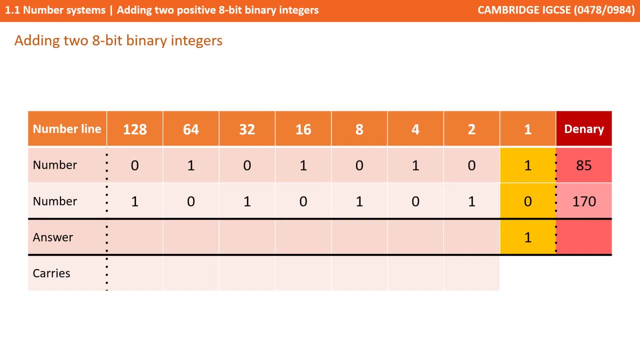 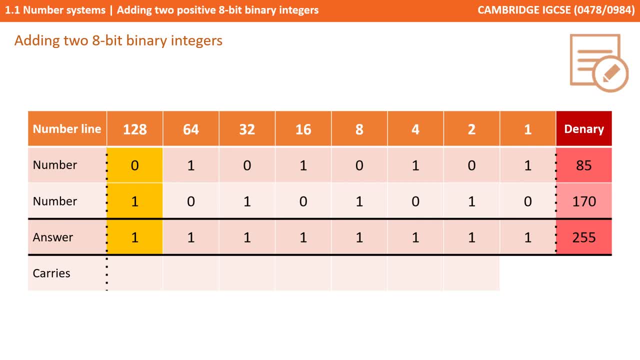 And a 0 plus a 1 is a 1.. A nice, simple, tidy, easy example. to start with, We add up every column that has a 1 in it, So that's all of them: 128 plus 60 plus 32, and so on. 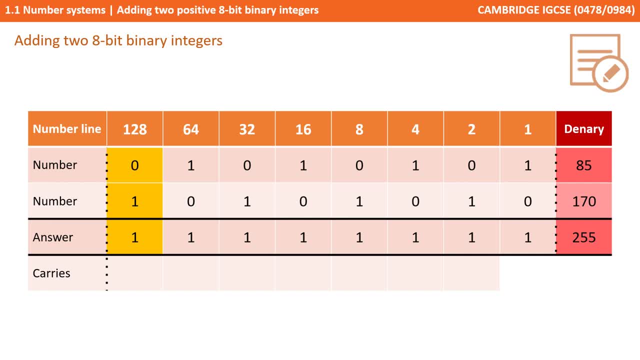 And we get 255, which, of course, is the original numbers 85 and 170 added together. OK, so let's take a look at another example, this time 43 plus 74.. So here I am again, and I've written out the two binary numbers. 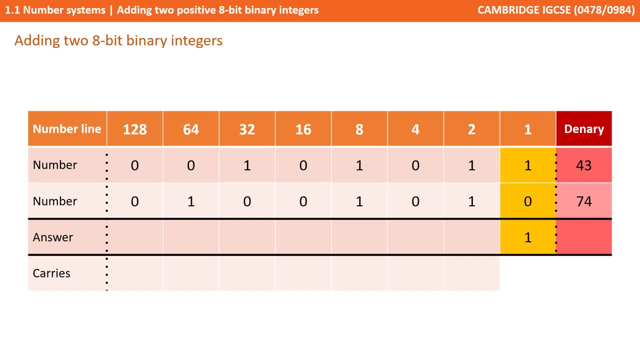 So let's start on the right. A 1 and a 0 is a 1.. A 1 and a 1 is a 0, and then we carry a 1 to the next column. It's important to show these carries in the exam. 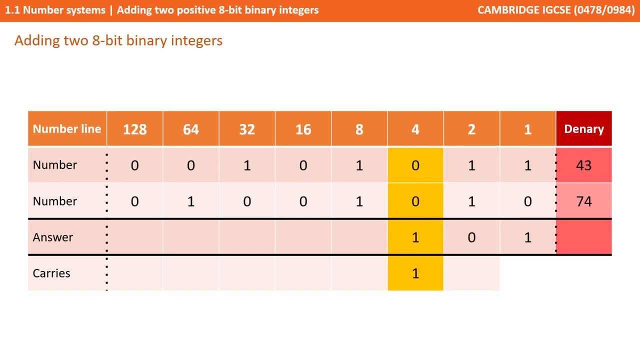 Write them underneath. So now we have a 0 and a 0, and the carry 1,. well, 0 and 0 and 1, is 1.. 1 and 1 is 0.. 0, carry the 1.. 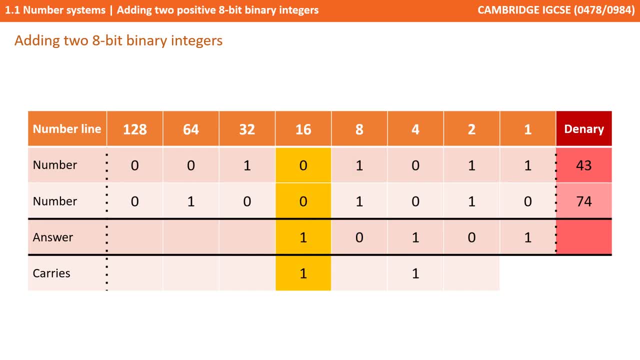 0, 0 and the carry 1 is 1.. 1 and 0 is 1.. 0 and 1 is 1. And 0 and 0 is 0. Again, you add up the columns that have the 1s in. 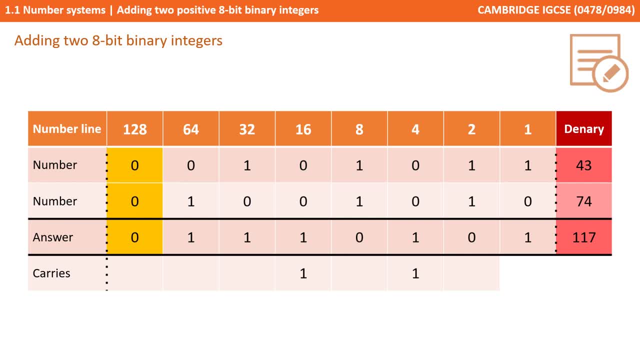 So that's a 64 plus a 32, plus a 16, plus a 4 and a 1, giving us 117.. OK, let's take one more example: 59. And then we'll have a 64 plus a 16 plus a 24.. 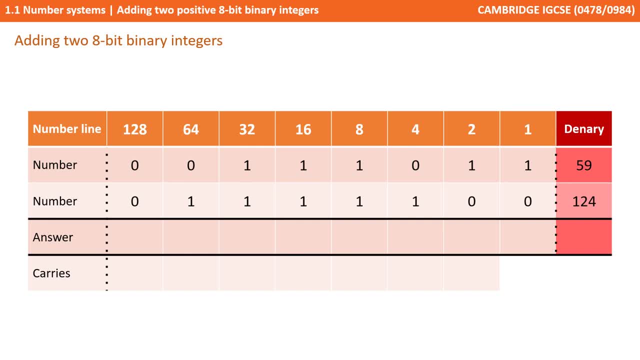 So again, I've written out their binary equivalents here Now. why don't you pause this video now and, on a scrap of paper, write down the binary edition and then unpause the video and see how you did So? a 1 and 0 is a 1.. 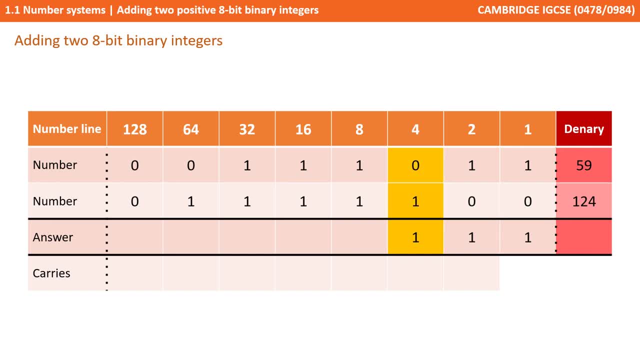 A 1 and 0 is a 1.. A 0 and 1 is a 1.. A 1 and 1 is 0, carry a 1.. A 1 and 1 is 0, carry a 1.. 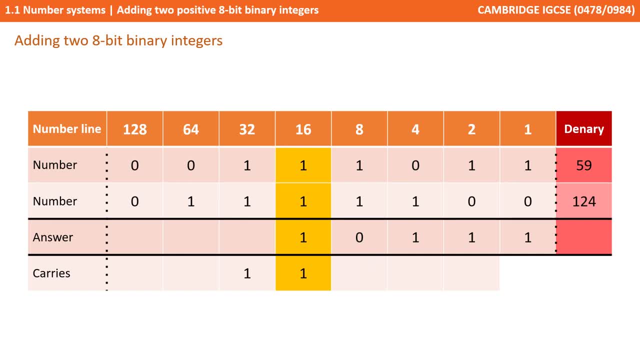 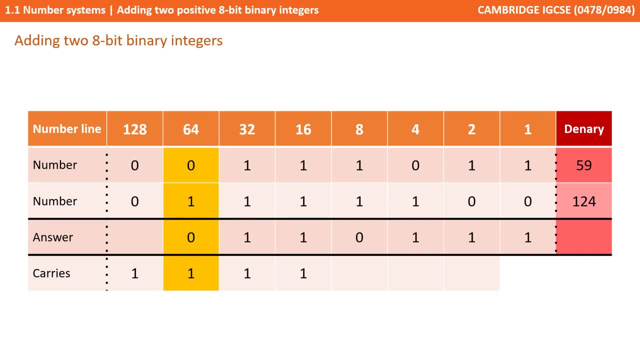 a zero one and the carry one is zero. carry the one and finally the zero zero and a carry one is one. so our binary answer is: one zero one, one zero one, one one which is 183. let's do one last example here. so we've got the numbers 95 and 222 in deanery. 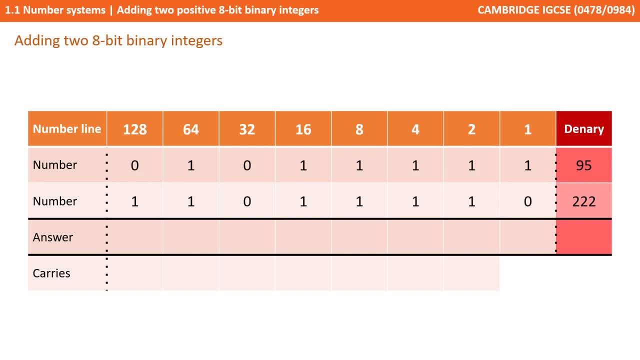 there they are written out under their binary waiting lines. again we start. on the right hand side we have one and zero. it's a one a one and one is a zero. carry a one, a one, one and a carry. one is one, carry a one. again we have a one, one and a carry. one is a one, carry a one. 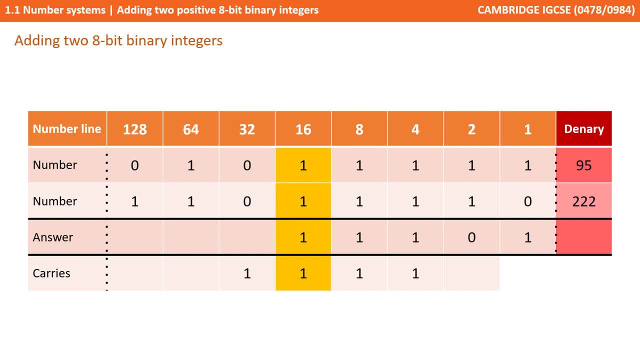 another one. one and a carry one is one, carry the one zero, zero plus a carry one is just one. one and one is zero. carry a one. and here we have a zero one and a carry one is zero and we need to carry an extra one, and what's happened here is we've got an overflow. our carry one is carry two, carry two 응. 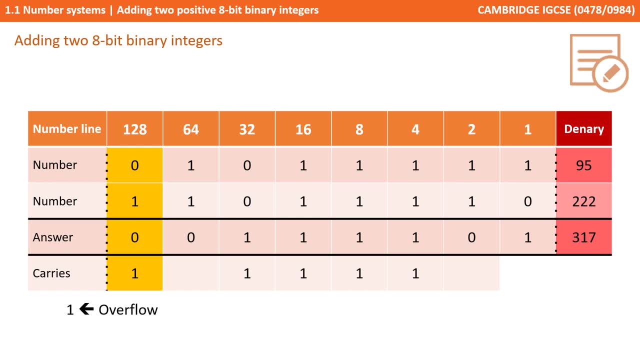 one has gone beyond the capacity of our current storage line and this is something which might crop up in the exam. The deanery numbers 95 plus 222 should equal 317, but if we read back the number we've actually got, we've got a 1 in the 32 column, a 1 in the 16 and 8,, a 4 and a 1. 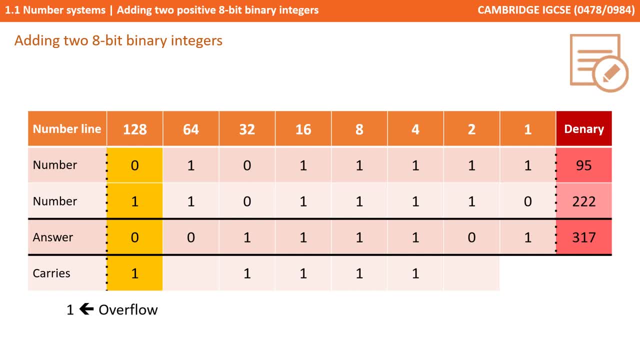 and that does not equal 317.. You might have spotted the reason for that. that's because the deanery number 95 can be stored in an 8-bit binary waiting line and the deanery number 222 can be stored in an 8-bit binary waiting line, but the sum of those two numbers 317.